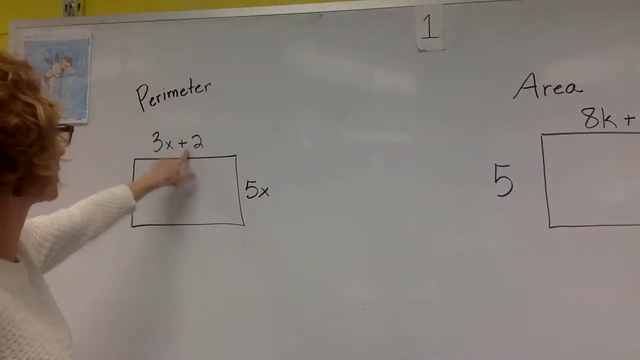 given a rectangle and I have a length that's 3x plus 2 and a width that is 5x. remember that perimeter means addition of all of the sides. So in this problem, if this visual was given to me, I would add to the visual and I would write down what the length is, based on knowing opposite sides. 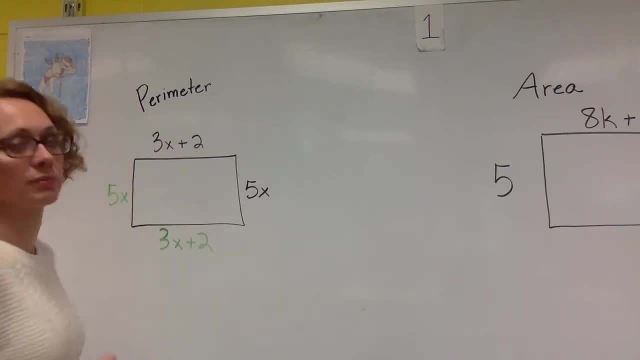 of a rectangle are congruent. That's the way I would make it look. So anytime I'm dealing with perimeter, I would think about addition of all of the sides. So here's what I'm going to write out: to find the perimeter. 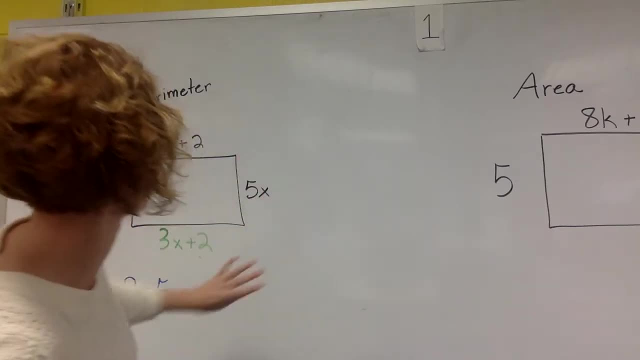 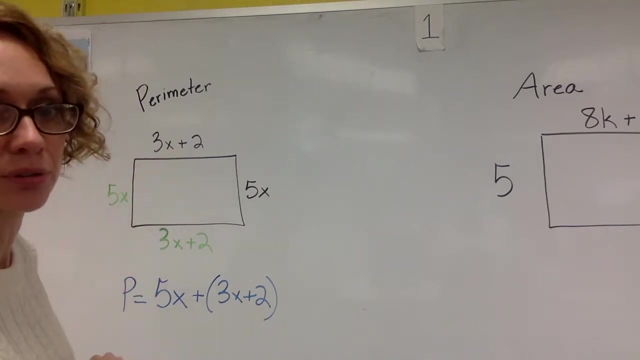 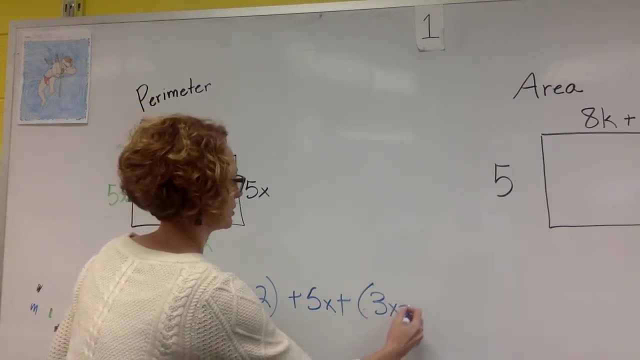 I usually start on the perimeter. I'm going to start on the left side of my shape and I go clockwise around it, So I'll plug in 5x plus 3x plus 2.. Notice, I'm putting that length in parentheses down there: Plus 5x plus this length, which is 3x plus 2.. 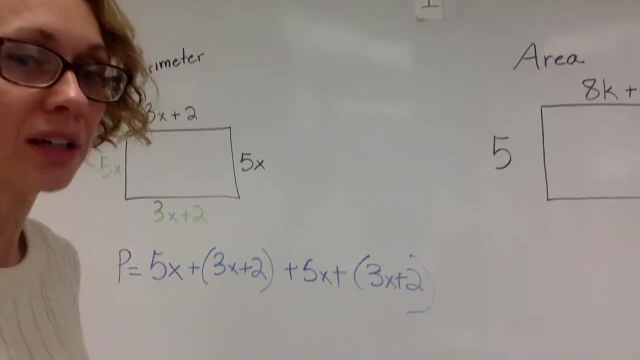 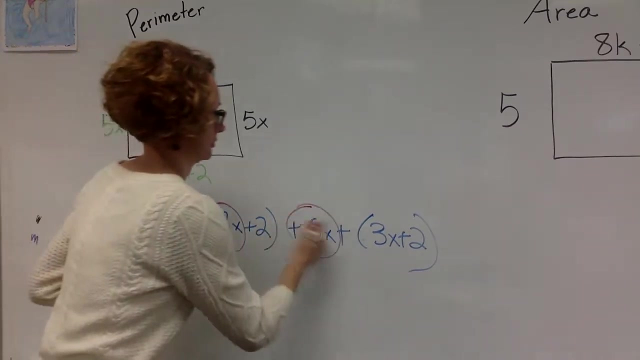 So, in order to get that perimeter completely simplified, what I'm going to do is I'm going to go through and identify my like terms. I'm going to circle All my x values and add them together: 5 plus 5 is 10, 3 plus 3 and. 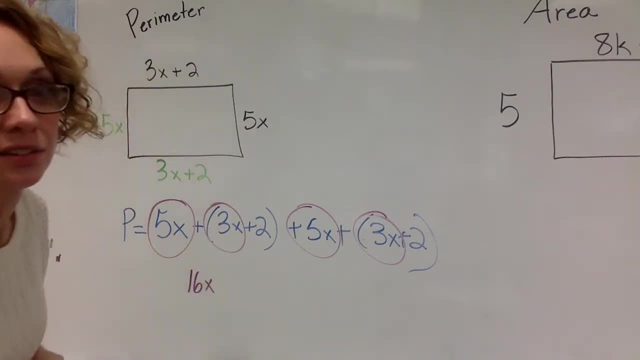 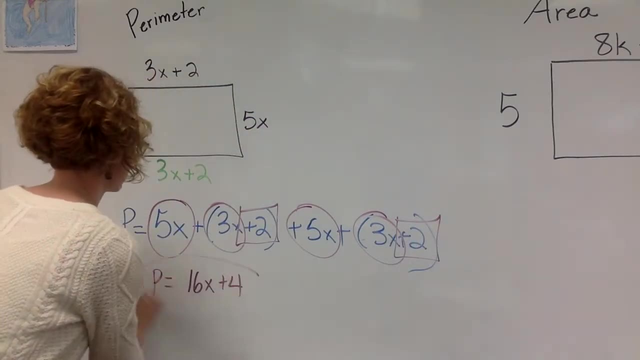 6, so that gives me a total of 16x, And then I'm going to put my numerical values together and that would give me four. So that's the way I'm going to write my perimeter. My final perimeter is left as an algebraic expression, and I'm OK with that as an algebraic thinker. 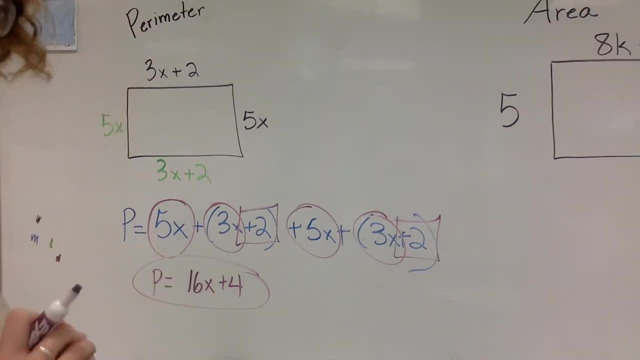 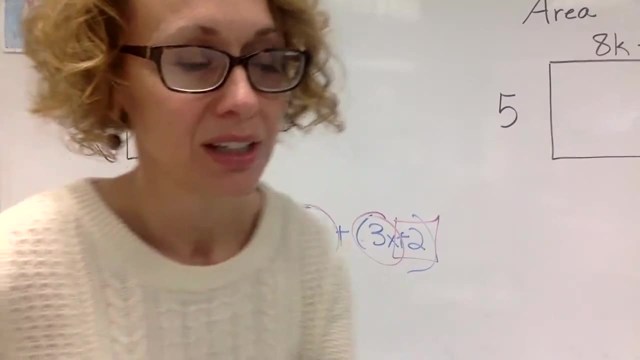 16x plus 4.. okay, so that's an idea of perimeter. no matter what the shape is that you're given for perimeter, remember you're gonna be adding all of the sides up. let's compare that to a problem that is dealing with area of geometric shape. so 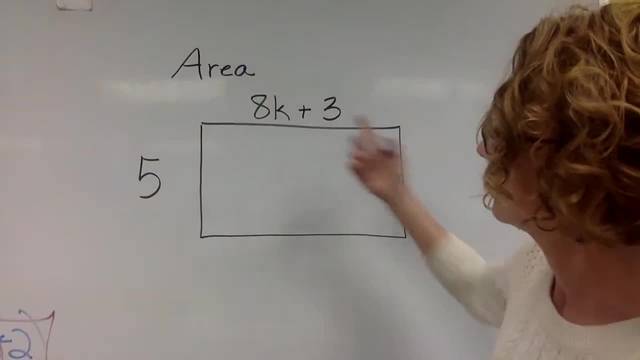 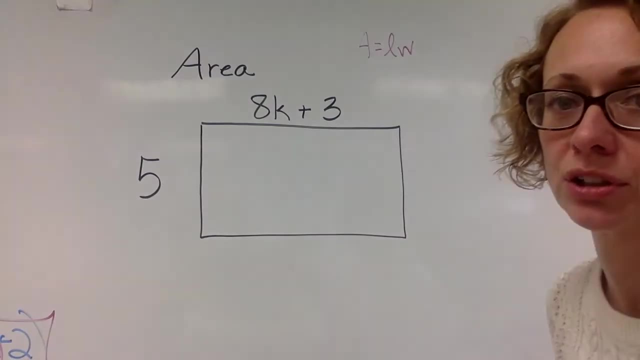 if I have a rectangle and it says, all right, find the area of this one. I know that the area formula for a rectangle is length times the width, so I'm gonna use that. I'm even gonna go over here to the side and I'm actually gonna start with. 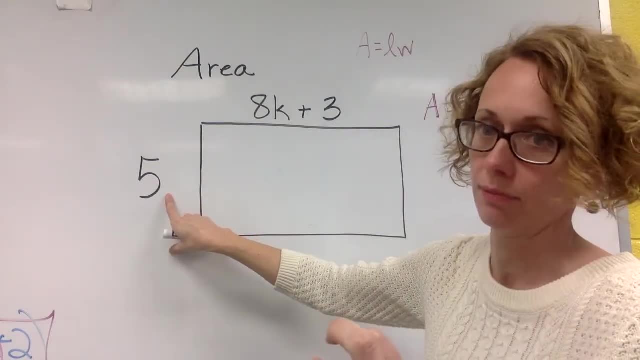 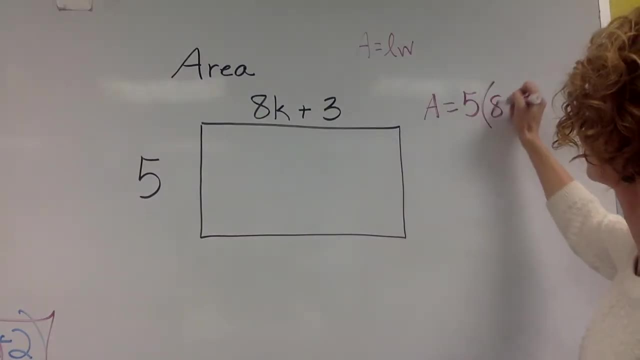 the width, because it's a monomial term. it's just a number and I'm gonna multiply that width times the length. look at how I'm gonna write that out. I'm gonna have 5 times 8 K plus 3 and I'm gonna use a distributive property to multiply that.